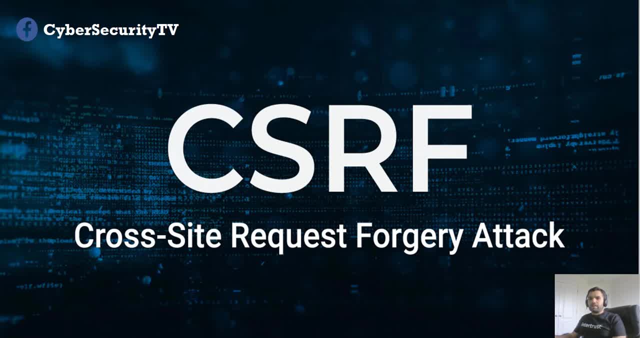 So I feel like since it has lost its rank in the US top 10,, people have not been paying attention to this vulnerability, but this is still fairly critical and that's what we're going to see today. And there are a lot of questions around CSRF because when I take interviews and I ask someone like what is the CSRF, they can't explain me confidently. They have good understanding of what the CSRF is, how you mitigate it and everything. 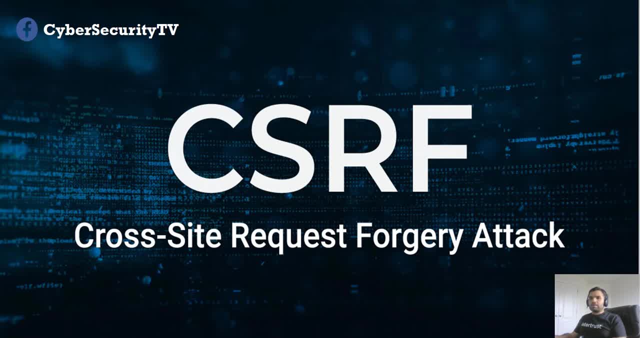 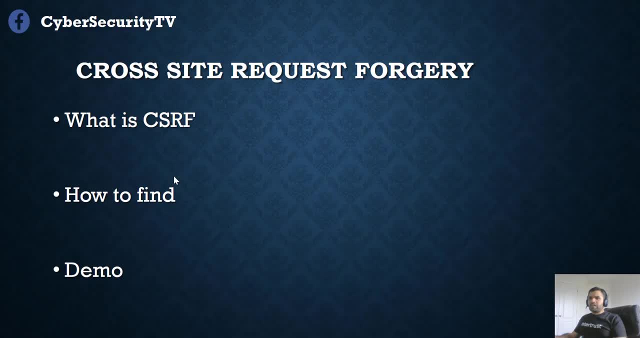 So I feel like since it has lost its rank in the US top 10, people have not been paying attention to this vulnerability, but this is still fairly critical and that's what we're going to see today. So I feel like since it has lost its rank in the US top 10, people have not been paying attention to this vulnerability, but this is still fairly critical and that's what we're going to see today. 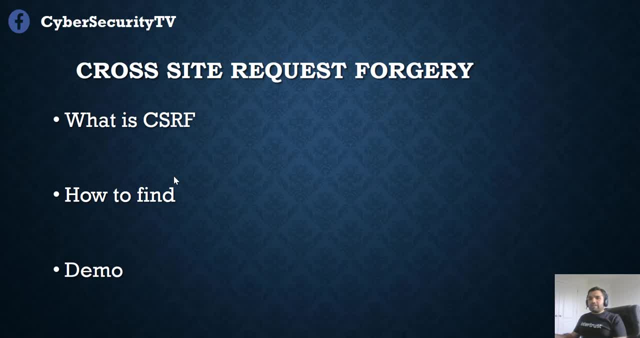 So I feel like since it has lost its rank in the US top 10, people have not been paying attention to this vulnerability, but this is still fairly critical and that's what we're going to see today. So I feel like since it has lost its rank in the US top 10, people have not been paying attention to this vulnerability, but this is still fairly critical and that's what we're going to see today. 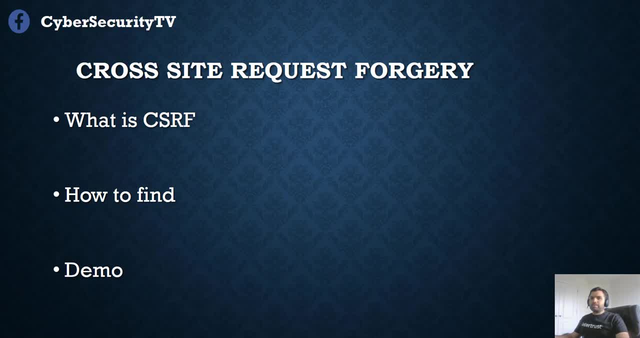 So I feel like since it has lost its rank in the US top 10, people have not been paying attention to this vulnerability, but this is still fairly critical and that's what we're going to see today. So I feel like since it has lost its rank in the US top 10, people have not been paying attention to this vulnerability, but this is still fairly critical and that's what we're going to see today. 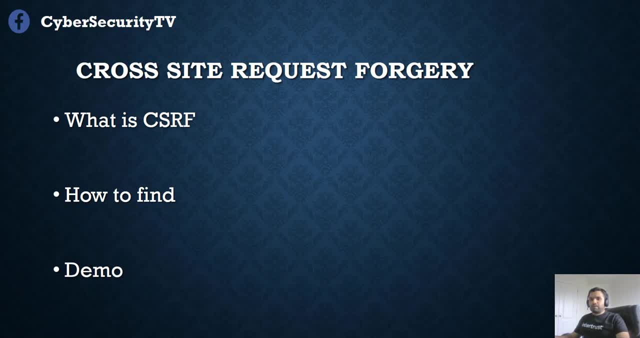 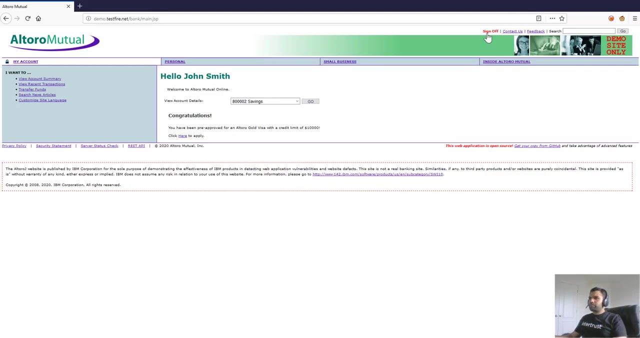 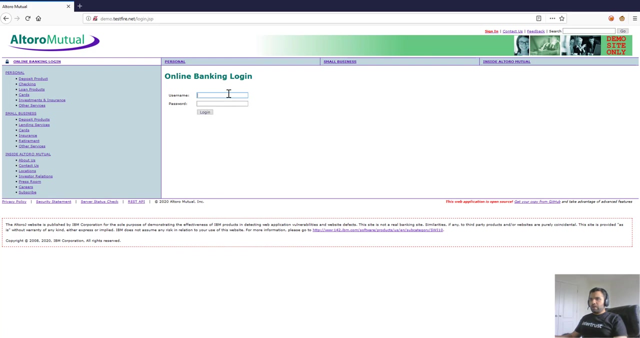 So I feel like since it has lost its rank in the US top 10, people have not been paying attention to this vulnerability, but this is still fairly critical and that's what we're going to see today. So I feel like since it has lost its rank in the US top 10, people have not been paying attention to this vulnerability, but this is still fairly critical and that's what we're going to see today. 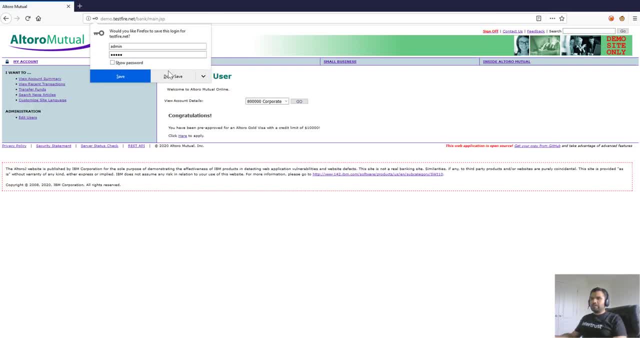 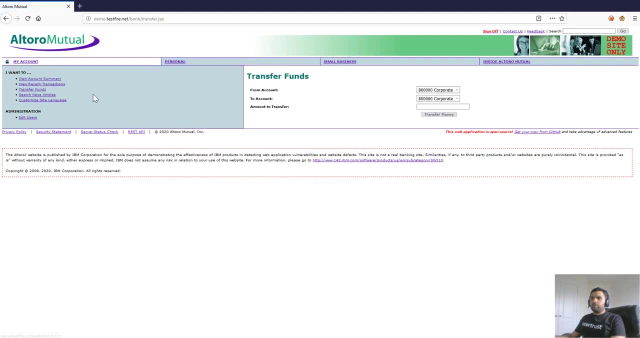 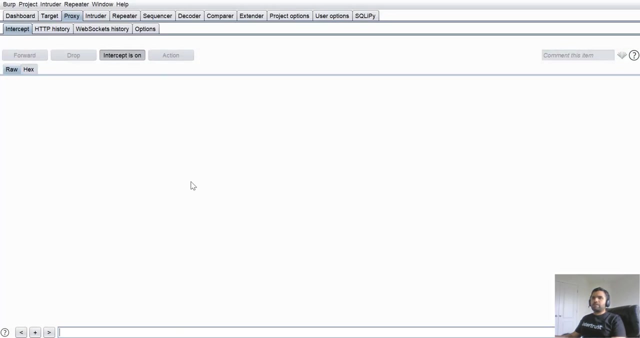 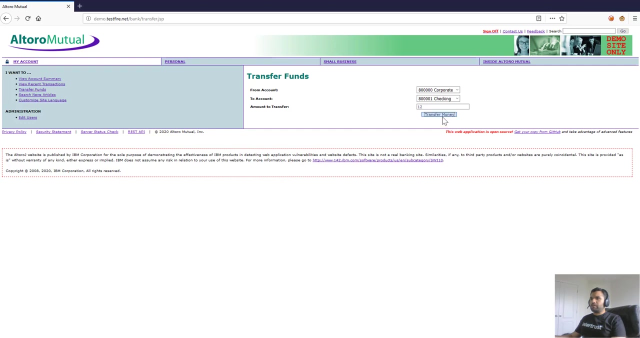 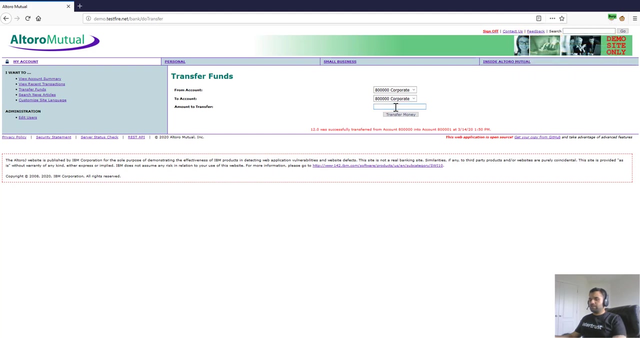 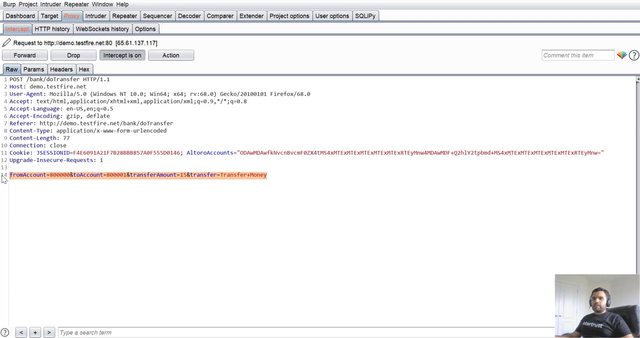 So I feel like since it has lost its rank in the US top 10, people have not been paying attention to this vulnerability, but this is still fairly critical and that's what we're going to see today. So I feel like since it has lost its rank in the US top 10, people have not been paying attention to this vulnerability, but this is still fairly critical and that's what we're going to see today. 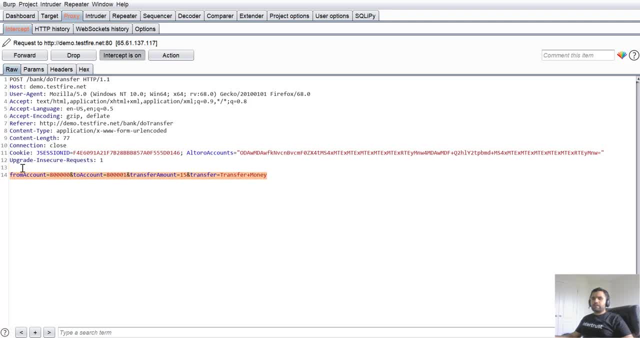 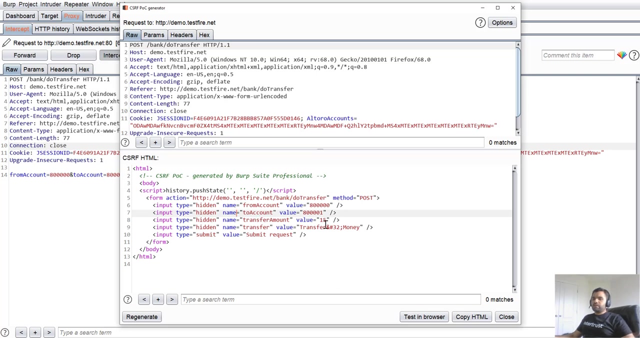 So I feel like since it has lost its rank in the US top 10, people have not been paying attention to this vulnerability, but this is still fairly critical and that's what we're going to see today. So I feel like since it has lost its rank in the US top 10, people have not been paying attention to this vulnerability, but this is still fairly critical and that's what we're going to see today. 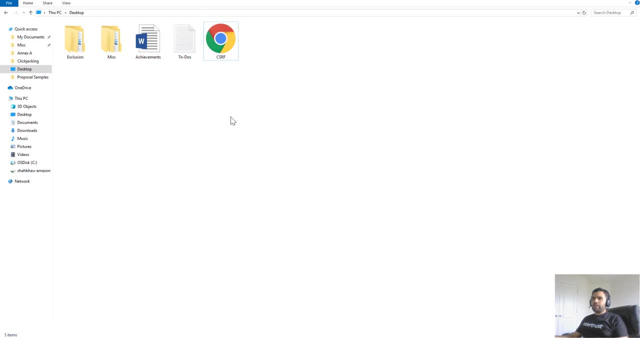 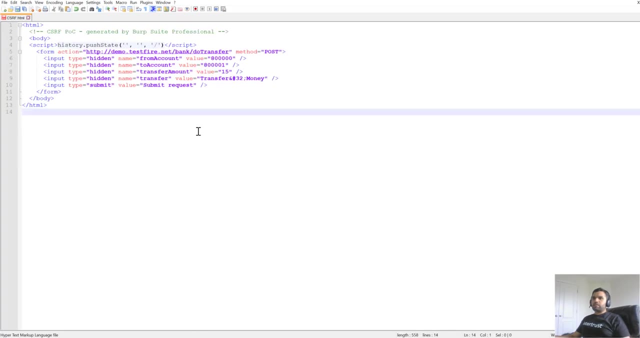 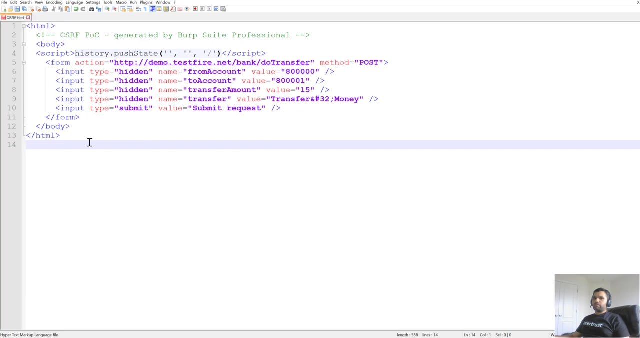 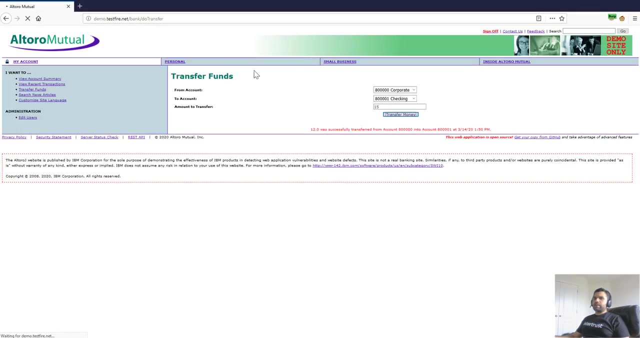 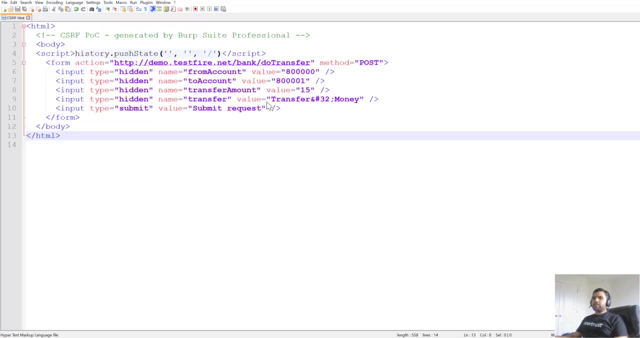 So I feel like since it has lost its rank in the US top 10, people have not been paying attention to this vulnerability, but this is still fairly critical and that's what we're going to see today. So I feel like since it has lost its rank in the US top 10, people have not been paying attention to this vulnerability, but this is still fairly critical and that's what we're going to see today. 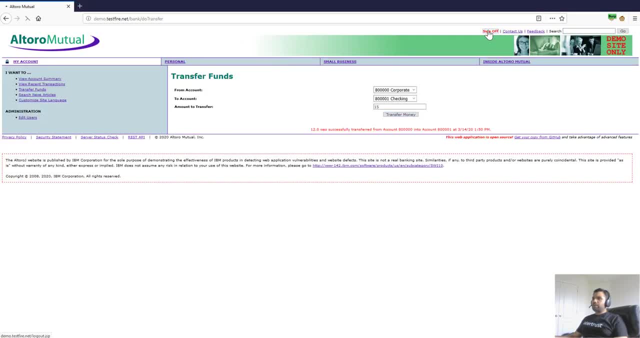 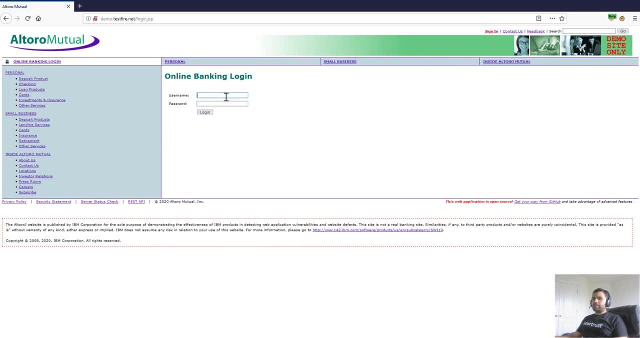 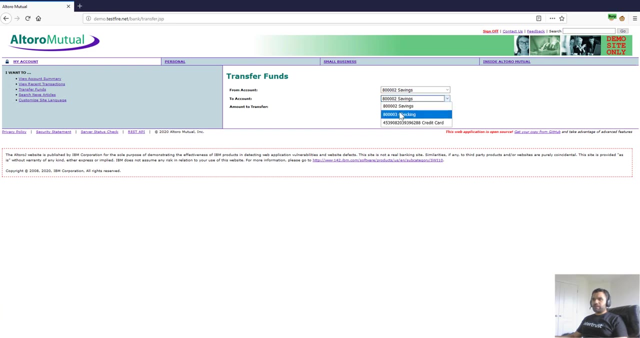 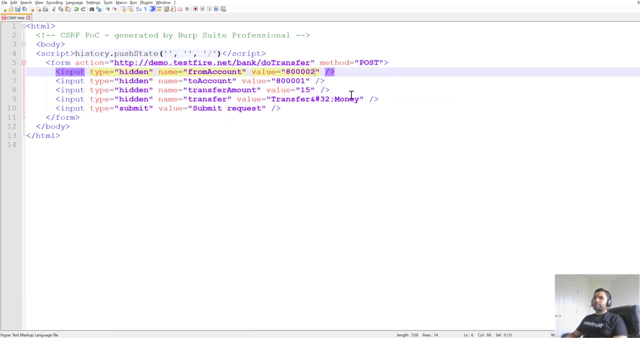 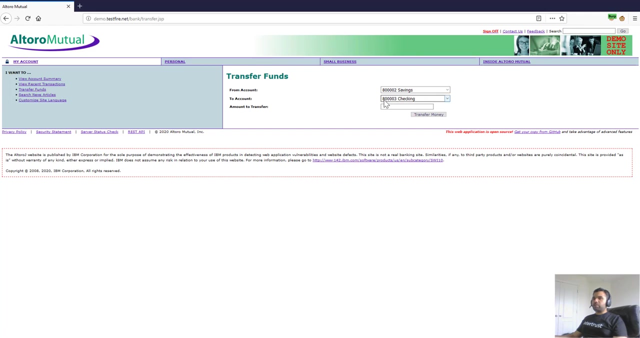 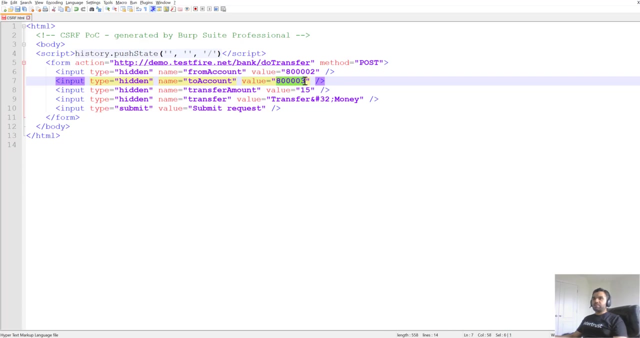 So I feel like since it has lost its rank in the US top 10, people have not been paying attention to this vulnerability, but this is still fairly critical and that's what we're going to see today. So I feel like since it has lost its rank in the US top 10, people have not been paying attention to this vulnerability, but this is still fairly critical and that's what we're going to see today. 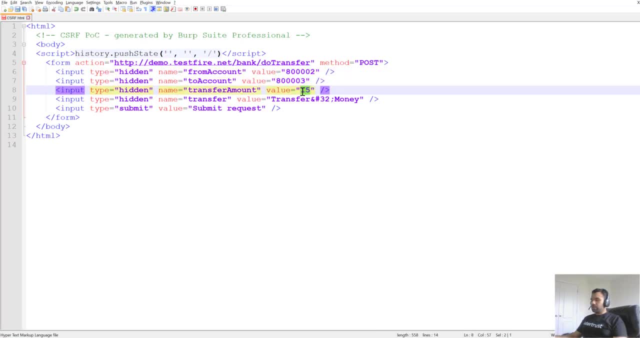 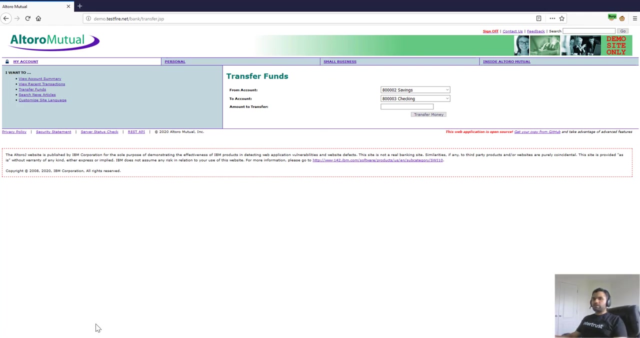 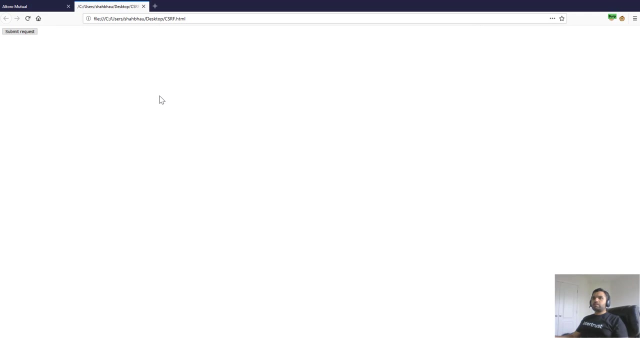 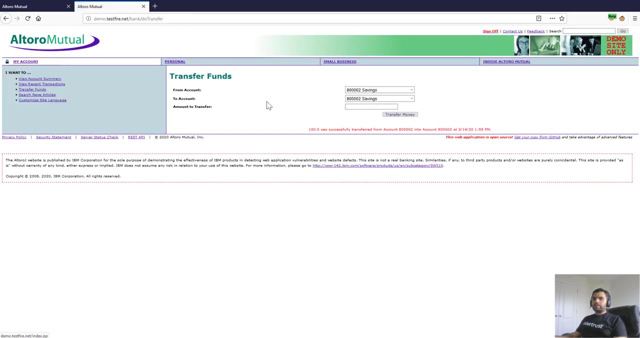 So I feel like since it has lost its rank in the US top 10, people have not been paying attention to this vulnerability, but this is still fairly critical and that's what we're going to see today. So I feel like since it has lost its rank in the US top 10, people have not been paying attention to this vulnerability, but this is still fairly critical and that's what we're going to see today. 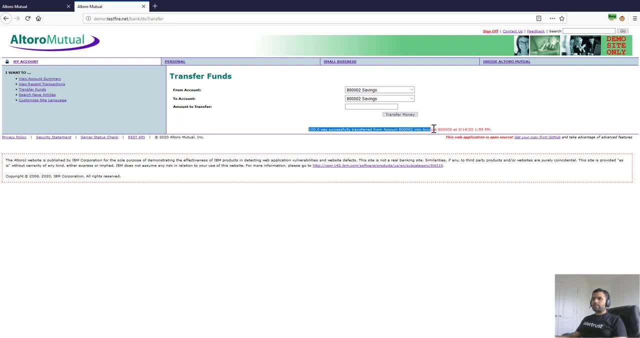 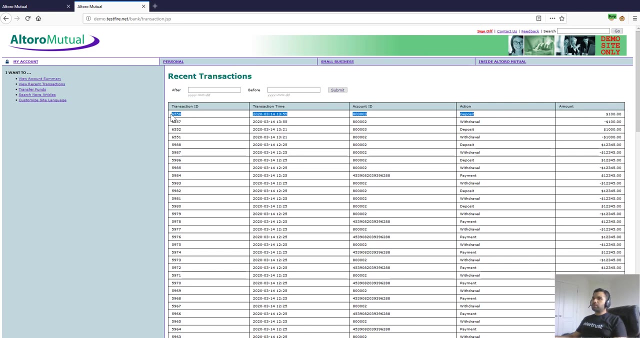 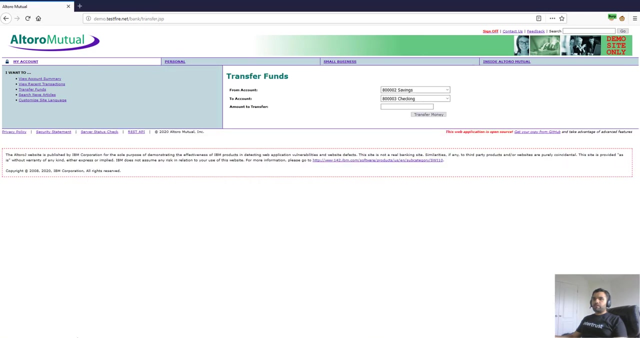 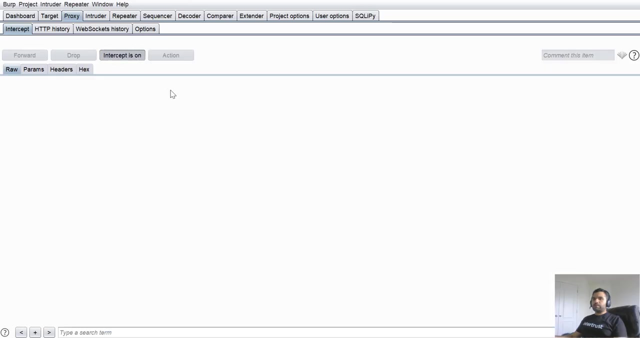 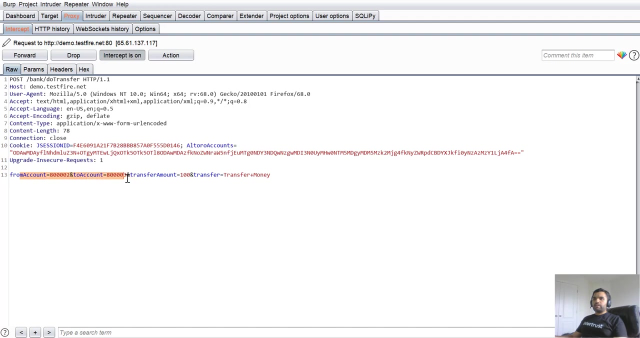 So I feel like since it has lost its rank in the US top 10, people have not been paying attention to this vulnerability, but this is still fairly critical and that's what we're going to see today. So I feel like since it has lost its rank in the US top 10, people have not been paying attention to this vulnerability, but this is still fairly critical and that's what we're going to see today. 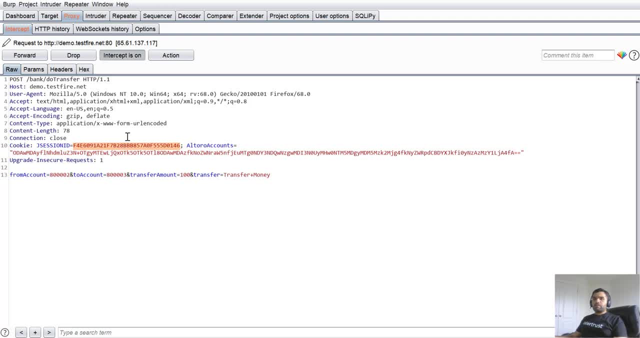 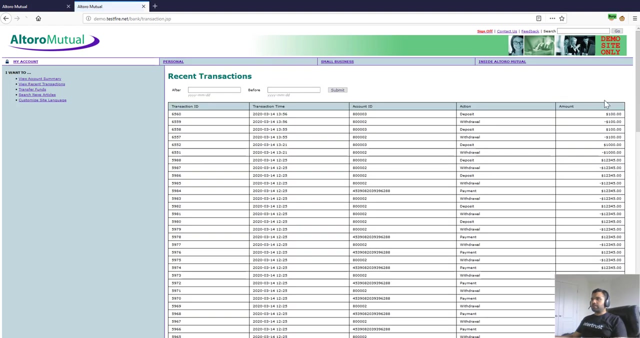 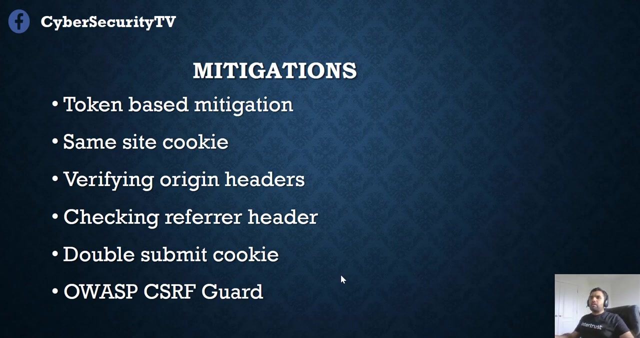 So I feel like since it has lost its rank in the US top 10, people have not been paying attention to this vulnerability, but this is still fairly critical and that's what we're going to see today. So I feel like since it has lost its rank in the US top 10, people have not been paying attention to this vulnerability, but this is still fairly critical and that's what we're going to see today. 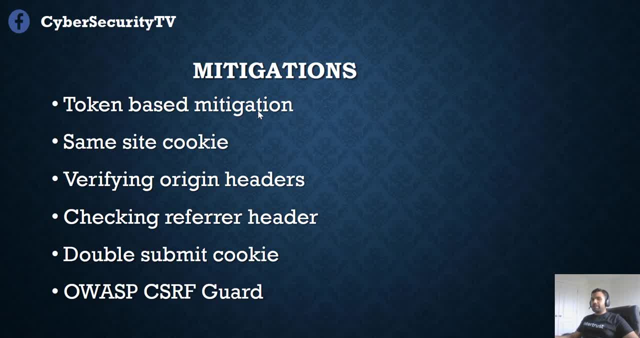 So I feel like since it has lost its rank in the US top 10, people have not been paying attention to this vulnerability, but this is still fairly critical and that's what we're going to see today. So I feel like since it has lost its rank in the US top 10, people have not been paying attention to this vulnerability, but this is still fairly critical and that's what we're going to see today. 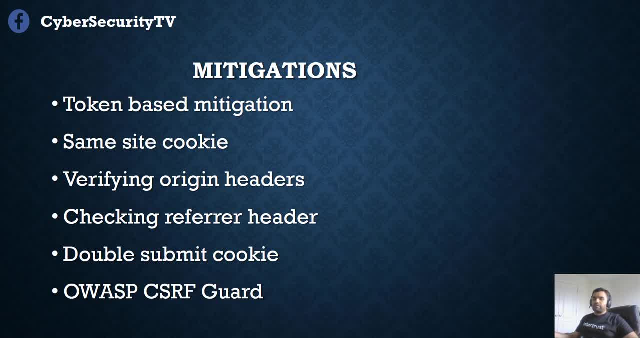 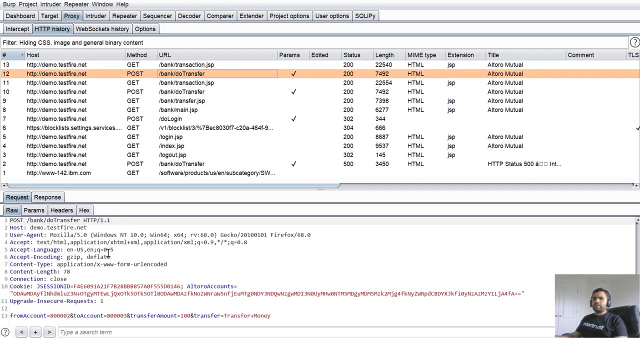 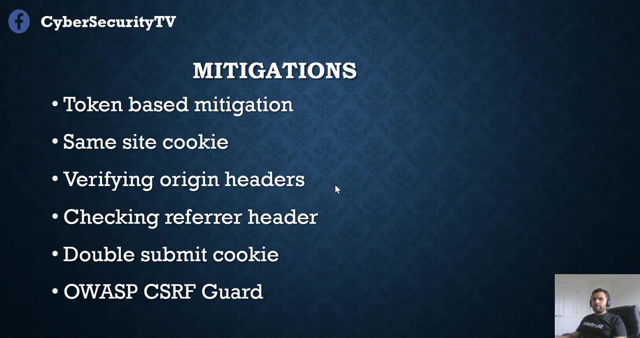 So I feel like since it has lost its rank in the US top 10, people have not been paying attention to this vulnerability, but this is still fairly critical and that's what we're going to see today. So I feel like since it has lost its rank in the US top 10, people have not been paying attention to this vulnerability, but this is still fairly critical and that's what we're going to see today. 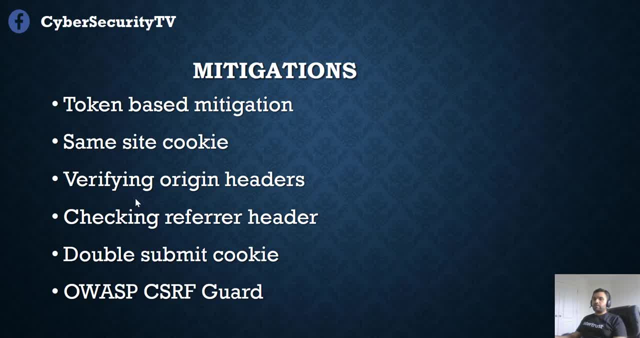 So I feel like since it has lost its rank in the US top 10, people have not been paying attention to this vulnerability, but this is still fairly critical and that's what we're going to see today. So I feel like since it has lost its rank in the US top 10, people have not been paying attention to this vulnerability, but this is still fairly critical and that's what we're going to see today. 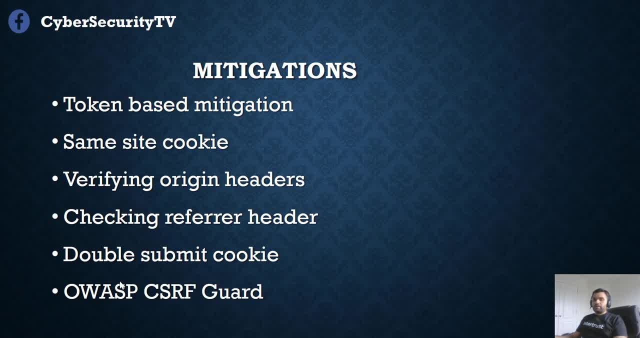 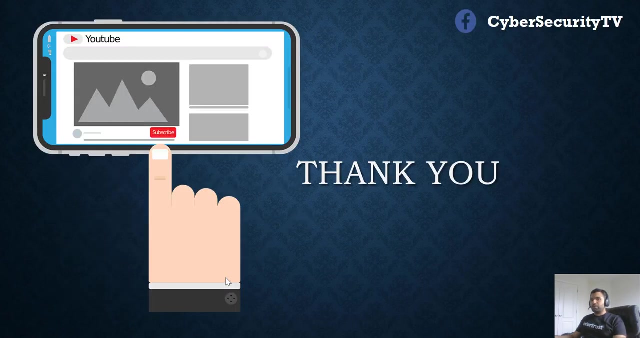 So I feel like since it has lost its rank in the US top 10, people have not been paying attention to this vulnerability, but this is still fairly critical and that's what we're going to see today. So I feel like since it has lost its rank in the US top 10, people have not been paying attention to this vulnerability, but this is still fairly critical and that's what we're going to see today. 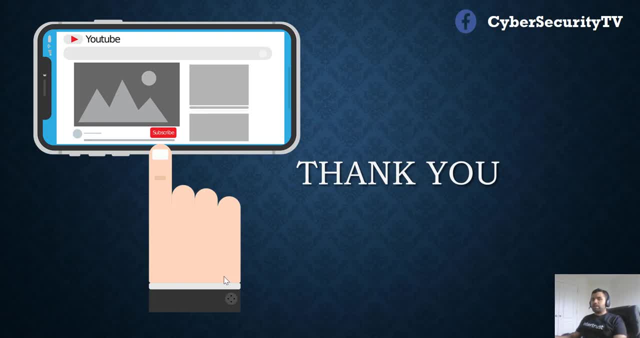 So I feel like since it has lost its rank in the US top 10, people have not been paying attention to this vulnerability, but this is still fairly critical and that's what we're going to see today. So I feel like since it has lost its rank in the US top 10, people have not been paying attention to this vulnerability, but this is still fairly critical and that's what we're going to see today. 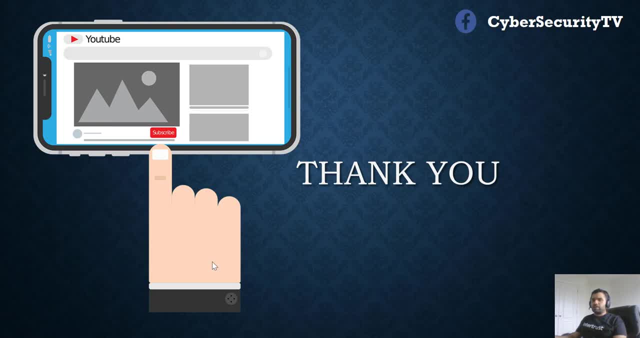 So I feel like, since it has lost its rank in the US top 10,, people have not been paying attention to this vulnerability, but this is still fairly critical and that's what we're going to see today. Thank you very much.